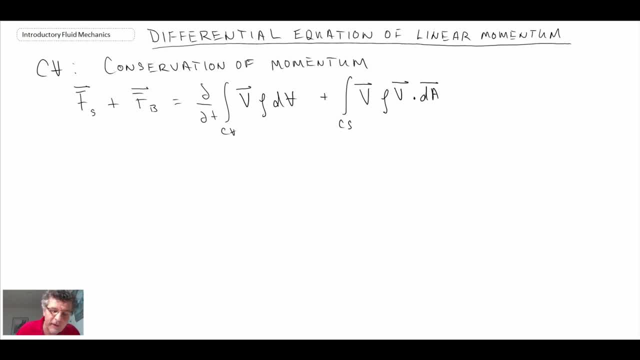 we're going to apply this, just like we did with continuity, to a little differential element and we'll say: the volume of that is dv, which is dx, dy, dz, the three dimensions of our little element, and consequently we can rewrite the conservation of momentum for that differential element. 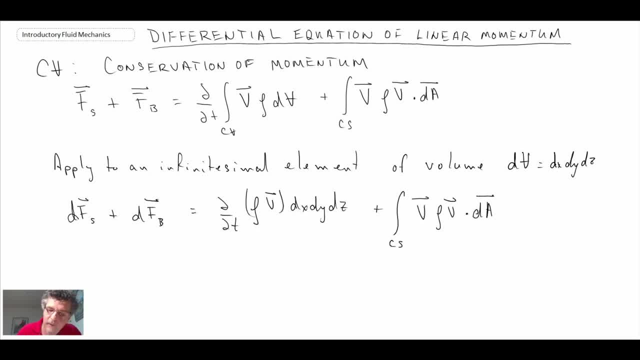 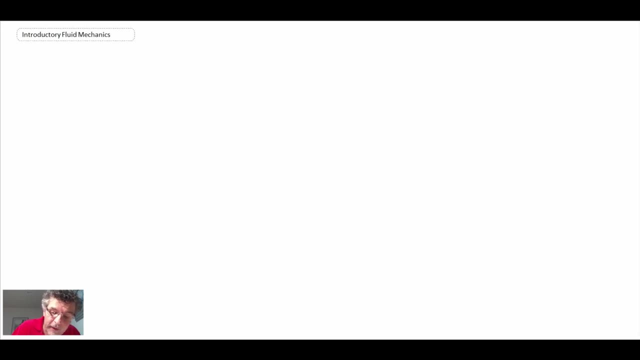 okay, okay, okay. so that's what we get, what we're now going to do. we're going to take this and we're going to look at the x momentum flux in the little differential element that we're interested in. so let me begin by writing a cube, drawing out a cube, and 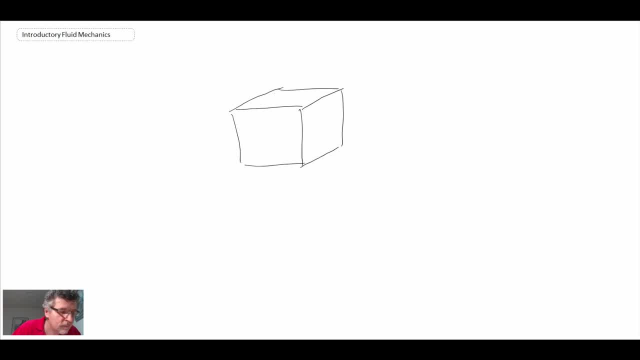 hopefully i'll put it in the middle this time. okay, so there is our little differential element, and what i'm going to do now is i'm going to sketch out momentum flux into the back surface and out of the front surface, so going in the x direction. 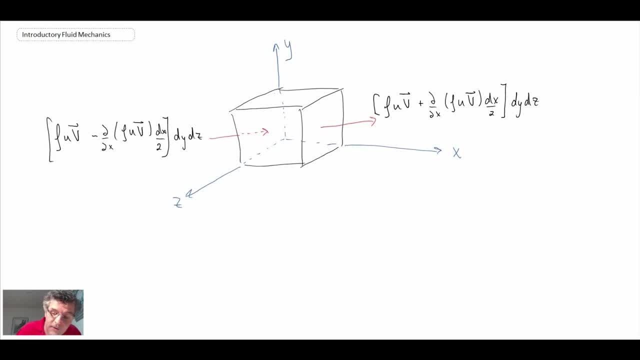 so there we have our momentum flux. i should have put here the size of the differential element. we have dx away, sorry, that should be be z z theلي, z z y n z, and then in the vertical we have dy. so that's the size, dimensions of our differential element. 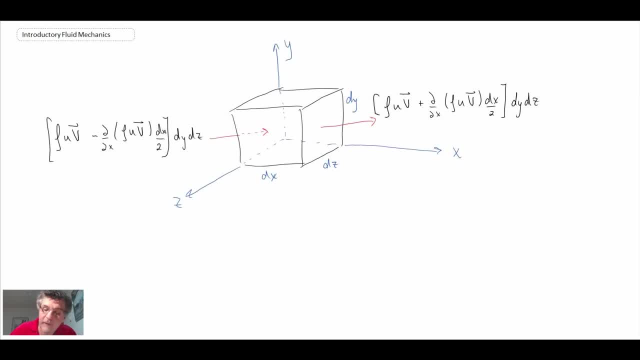 and what we have is momentum flux into the back and out the front, and we use the Taylor series expansion to do that. and in doing that, what we're doing is we're assuming that we are expanding about the midpoint of our little differential element. so what we're now going 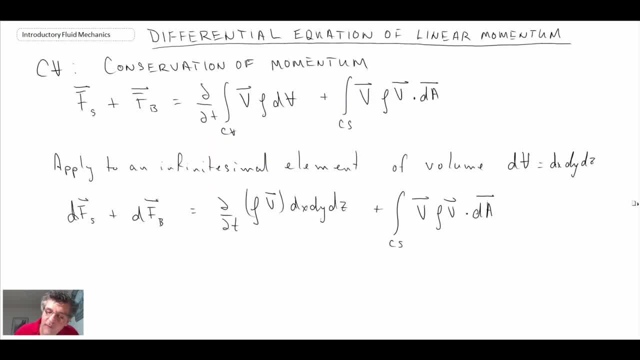 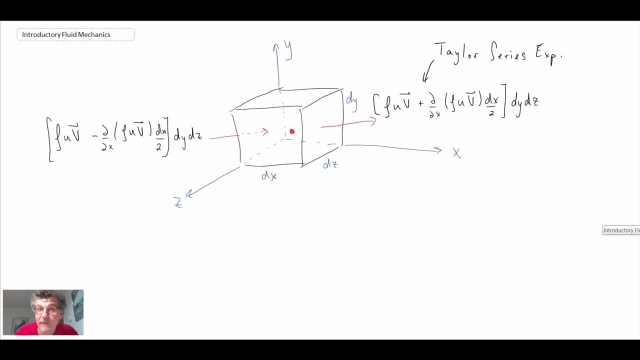 to do now? looking back at the momentum equation- we're going to play around with this term here- looking at the momentum flux into an out of our control volume. there is our control volume. we've written momentum flux in one direction, but we will have to expand that for all three directions. we're 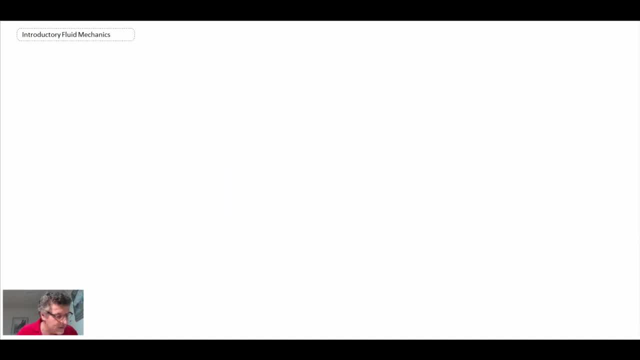 not going to do that. well, we will, but I'll show you the result. so, anyways, let's start with the momentum flux in the x direction and take a look at what that looks like. and again, just like all other control volume analysis we've been doing, we have to. 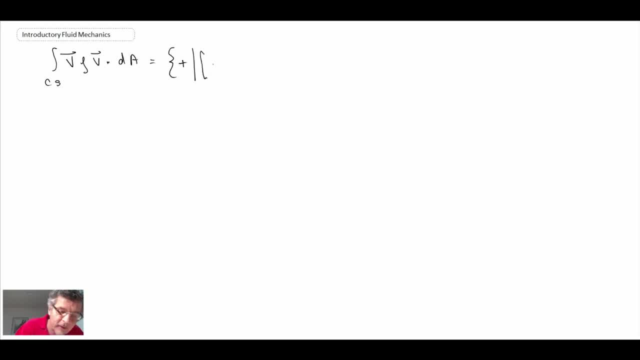 be careful about the sign of what is flowing in and what is flowing out, so that's flowing out of the right hand side and then coming in on the left hand side, we'll have a negative and just because the way the vectors work out with the dot product. 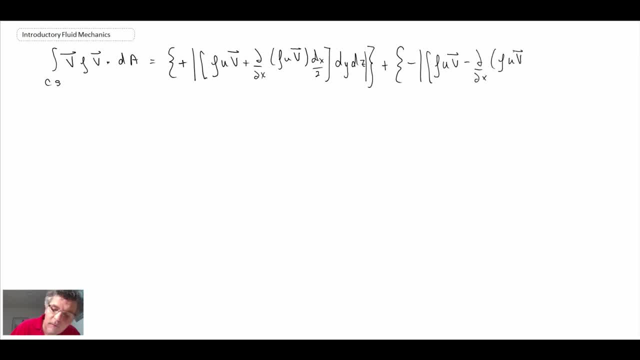 okay, and that's the area that it is flowing out over, and then we have plus y direction and then plus c direction. so if we go in and we perform this for all three directions and we add up terms and we cancel out, we have plus y direction and then plus. 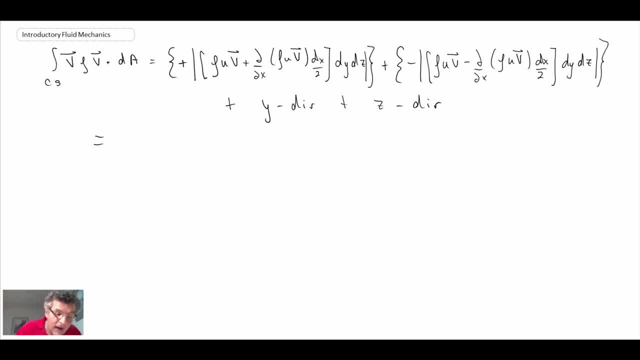 z direction and we do a bunch of different things like that. what we'll find is we get something that looks like the following: and that is then multiplied by dx, dy, dz, which is the volume of our differential element. So with that, what we can do is we can combine this with the first term on the right. 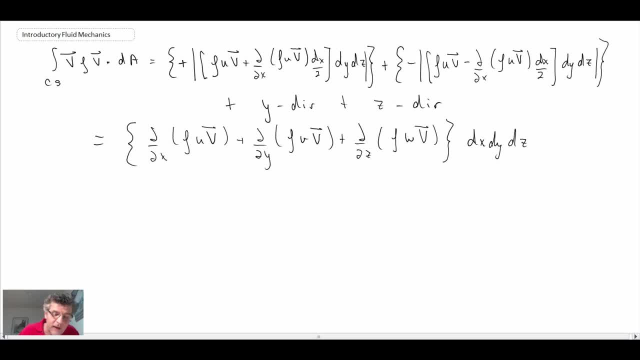 hand side of the control volume formulation And the left hand side is going to be our forces. So we have our surface forces plus our body forces, And then on the right hand side I'm going to pull that volume term up to the front And we get this.